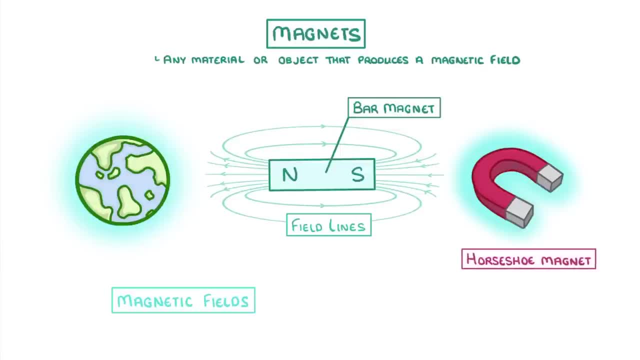 shapes and sizes, from these simple horseshoe magnets to the entire Earth itself, which is basically one huge magnet. What all magnets have in common, though, is that they have two poles, a north and a south, and they're surrounded by a magnetic field. 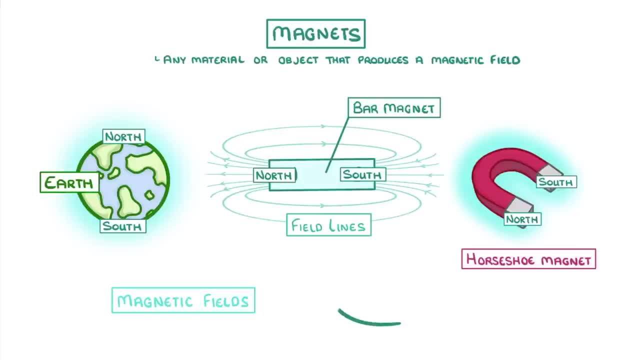 In order to properly represent these magnetic fields, we use something called field lines, which are effectively arrows that you draw around your magnet From the north pole to the south pole, And it's important that you can draw these lines for your exam and that you put the 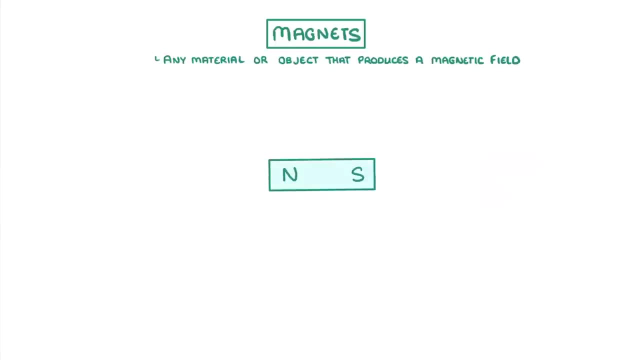 arrows in the right places. The easiest way to do this is to draw at least one straight line going into the south pole and coming out of the north pole, then a pair going into the south pole that are slightly curved, and a similar pair coming out of the north, and then, lastly, some that loop all. 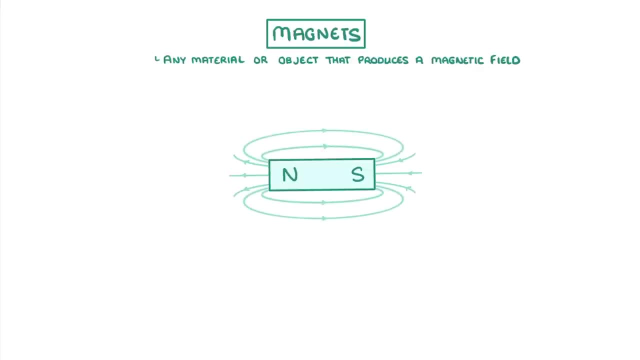 the way around from the north to south, As well as these basic lines. you could add in some more arrows if you want to, in the same style, but you generally don't need to for exams, And the last thing you want to do is double check that all of your little arrows are pointing. 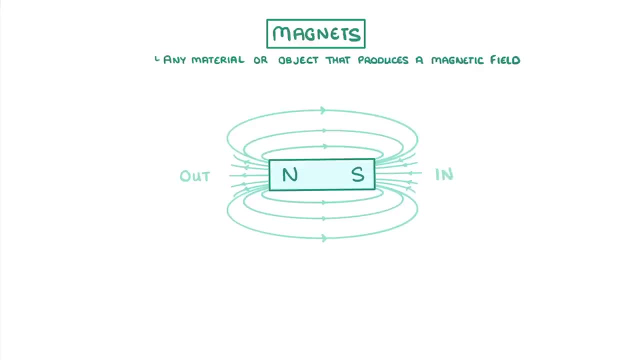 the right way, because we want our arrows to go out to the north and into the south. The benefit of representing our magnetic field with lines like this is not only that it shows us where the field is and which direction it's acting in, but that it also shows us. 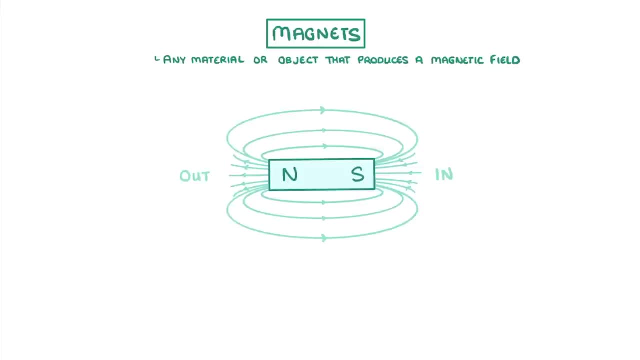 the relative strength of the field in different places, because the more dense the field lines are, which is to say the closer together the lines are, the stronger the magnetic field is in that area. For example, we can see that the field would be much stronger over here by the north pole. 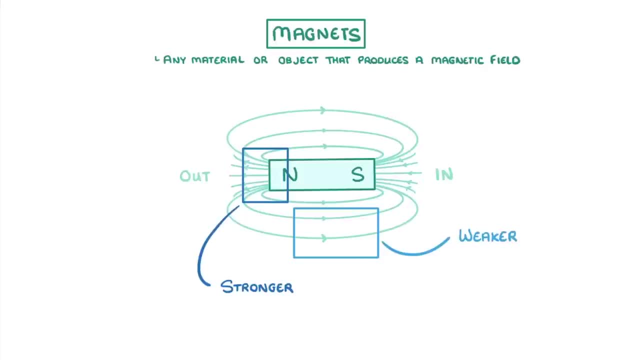 than it would out here to the side, because this one by the pole has lots more lines going through it. Now, in real life, we obviously can't see the field lines, and magnets aren't always labelled with a north and south. However, we can easily find the poles and field lines by using a compass.